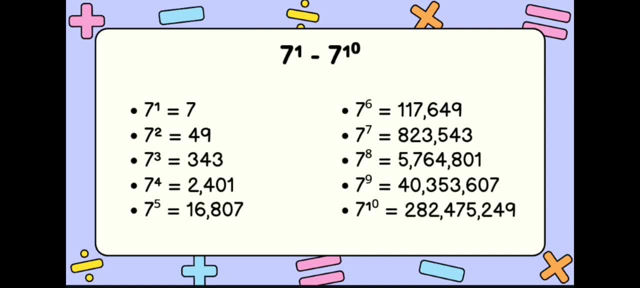 So 7 raised to 1 is 7.. 7 raised to 2 is 7.. 7 raised to 2 is 49.. 7 raised to 3 is 343.. 7 raised to 4 is 2,401.. 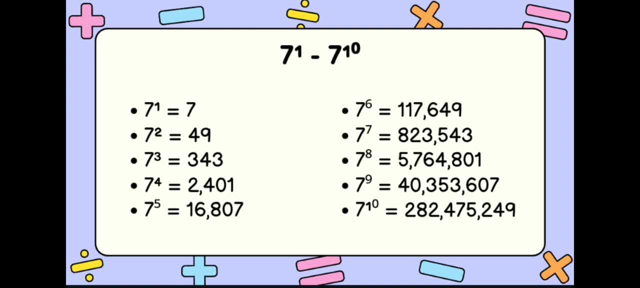 7 raised to 5 is 16,807.. 7 raised to 6 is 117,649.. 7 raised to 7 is 823,543.. 7 raised to 8 is 5,764,801.. 7 raised to 9 is 40,343. 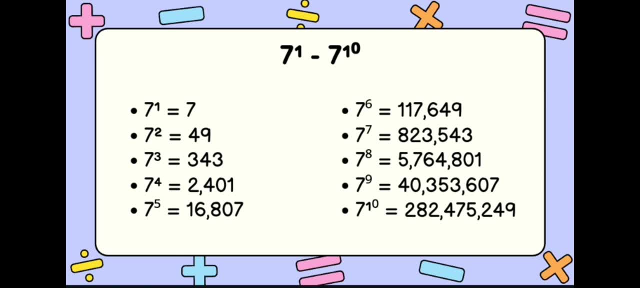 And 7, raised to 10, is 282,475,249.. So, as we can see, our rightmost digits, or unit digits, are repeating, So we have to simplify this and leave behind the unit digits. So, as we can see, we have 7,931 as our unit digits. 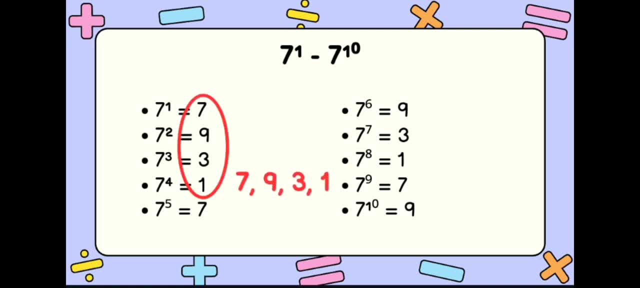 So we have this 7,931.. So we have 4 digits. So our next step is we will be dividing the exponent to the total number of the repeating digits. So 146 divided by 4.. So the quotient is 36.2.. 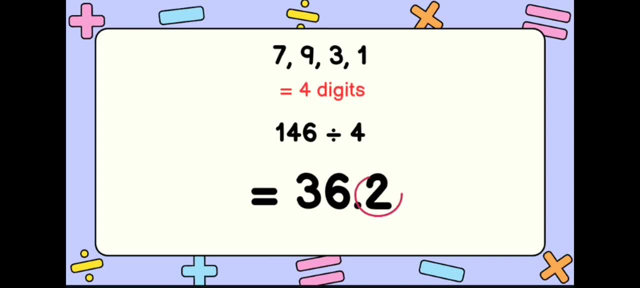 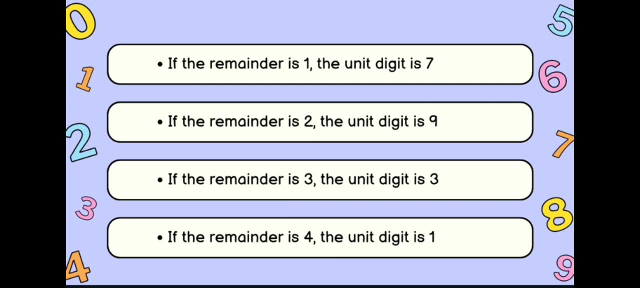 So we will get the remainder, which is 2.. Next is, we will get the unit digit through the remainder. So if the remainder is 1, the unit digit is 7.. If the remainder is 2,, the unit digit is 9.. 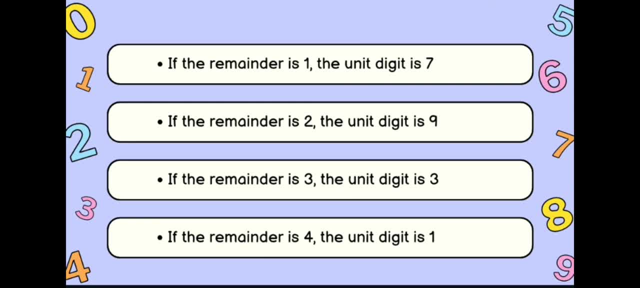 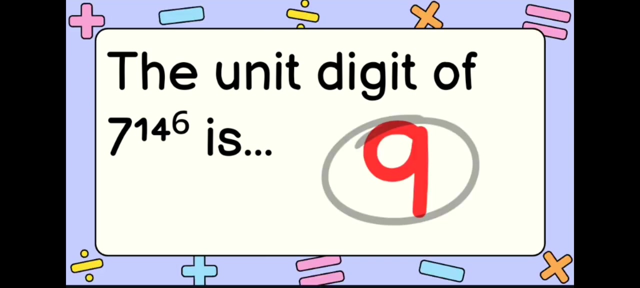 If the remainder is 3,, the unit digit is 3.. And if the remainder is 4,, the unit digit is 4.. So which one of these is our answer? You got it right. Our remainder is 2.. Therefore, the unit digit of 7 raised to 146 is 9.. 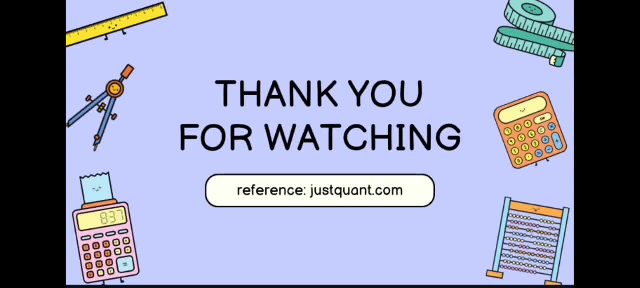 And that is all for determining the unit's digit. Thank you for watching.